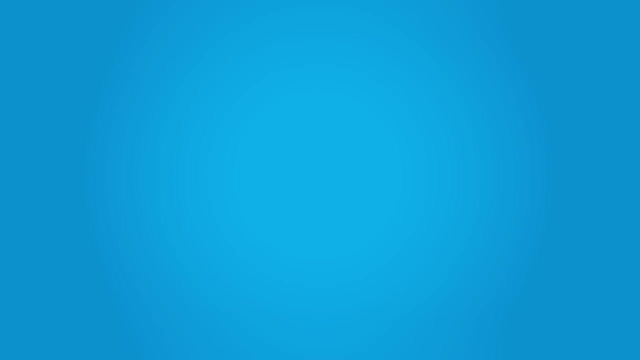 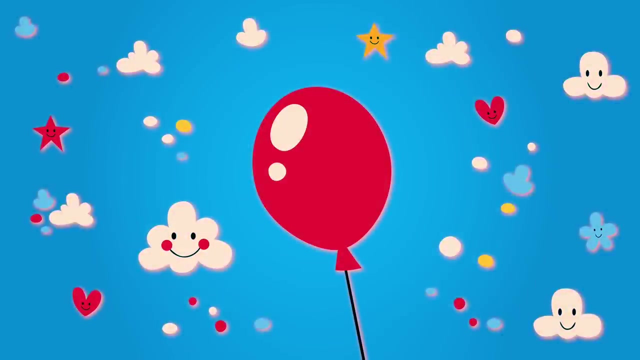 Please add punctuation in the appropriate places And either lie down on your back side or tummy or sit cross-legged or on a chair. Take a moment now to decide which works best for you. Now you've found your spot, have a wriggle and a fidget so your body feels happy. 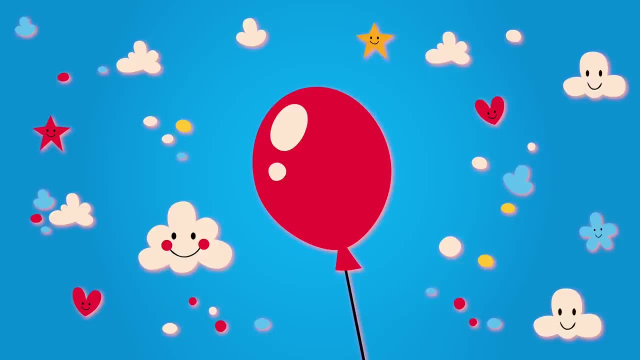 And when you're done, say goodbye to those fidgets And hello And hello to that lovely, warm, calm feeling you get when you're relaxed and your body comes to stillness, Rest and breathe gently. You can keep your eyes open for now if you like. 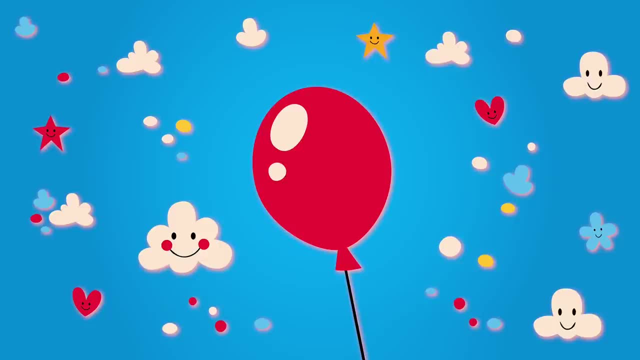 See if you can feel your breathing. You might need to slow it down a little so you can feel what it's doing to your tummy, Making it lift as you breathe in and lower as you breathe out. Next time, as you breathe out. 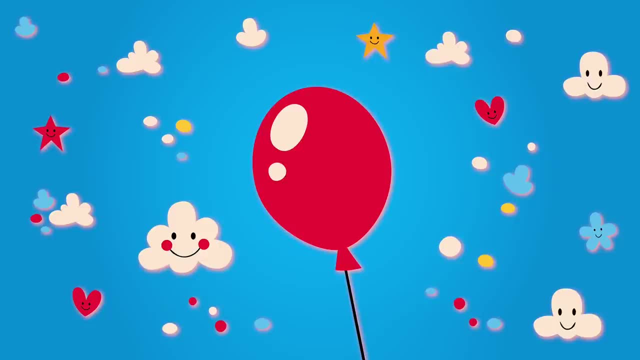 let your eyes softly close. Well done. Now you can enjoy the adventure With your eyes closed. your mind can make the pictures for you. You are outside in a garden And up in the sky you spot a red balloon floating. You can see it has a little string dangling down. 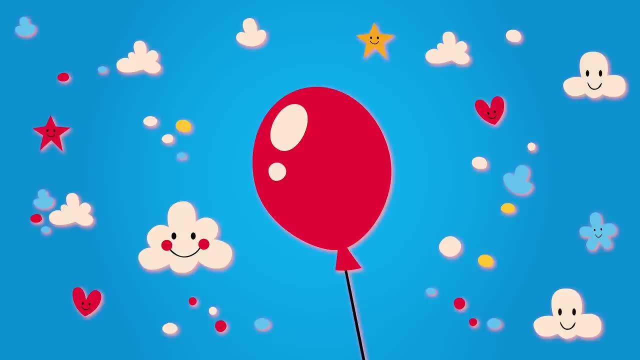 It's floating down towards you. You wonder why. You wonder why. You wonder where this balloon has come from And why is it here for you Now? it is right in front of you, Like it's waiting for you to take it. 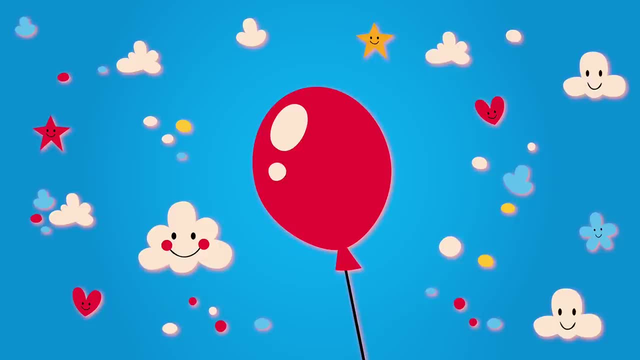 You reach your hand forward and take hold of the string. Now you feel the balloon start to rise again up into the sky. You don't let go And you feel it pulling you up too. It lifts you right up onto your tiptoes. 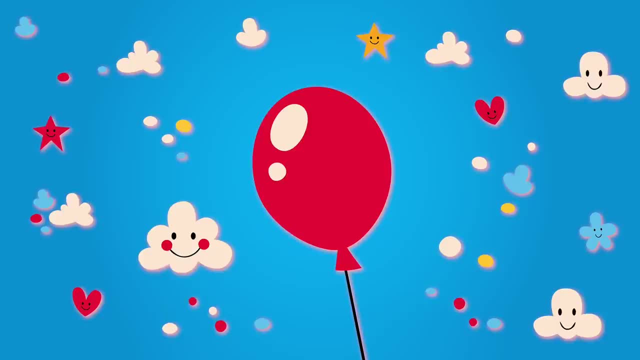 And then your feet leave the ground And you are floating too, Just like the balloon. Where are we going, you wonder. You relax, You relax And let yourself be carried, Enjoying the cool air on your skin. You see green fields down below. 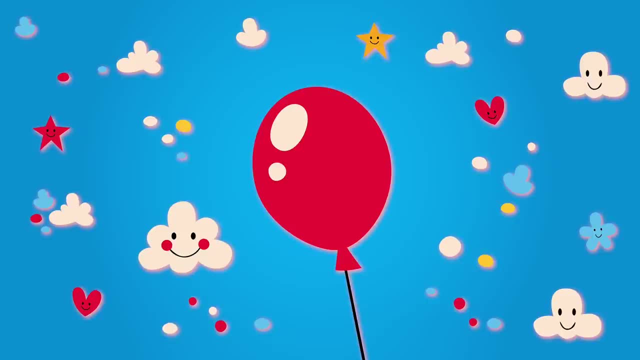 And the trees. You are above the treetops Looking down on them. Look Just up ahead. You see your favourite place in the whole world. You decide what this place is. See if you can imagine it now. What does it look like? 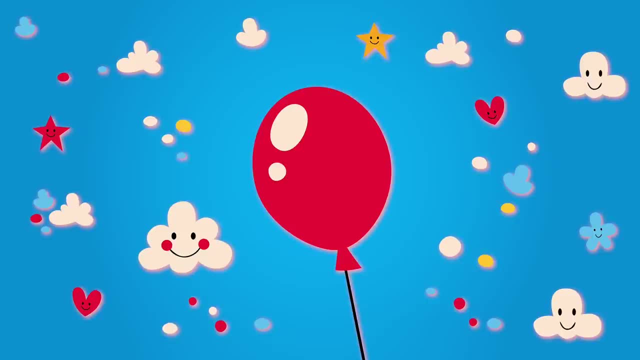 The balloon takes you right to it And you are lowered gently. So you and the balloon are there. now Look around at this place. What can you see? Can you hear any sounds? Are there any people here Or animals? Or is this a place you enjoy all by yourself? 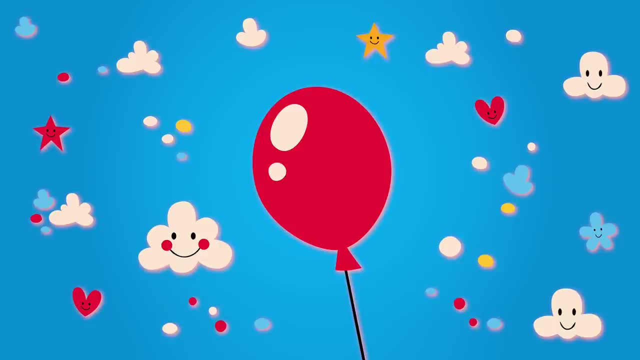 Does it have a particular smell Or taste? maybe, As you stand here with your red balloon, you soak up the goodness and joy from being here in your favourite place, How much you love it, Breathe into it As you do. you feel completely happy.